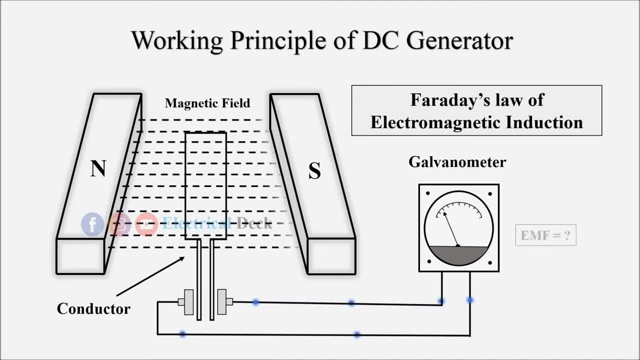 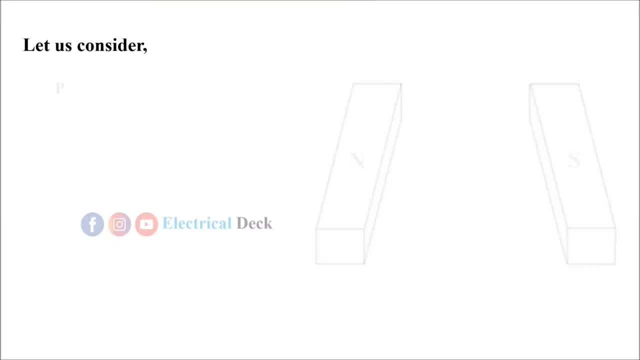 Let us check out and derive an equation for amount of EMF produced by the generator. Let us consider: P is equal to number of poles of the generator. P is equal to amount of flux produced by each pole in Weber. N is equal to speed of armature rotating in rpm. 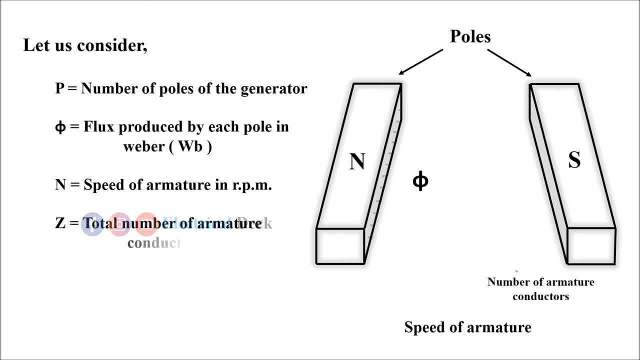 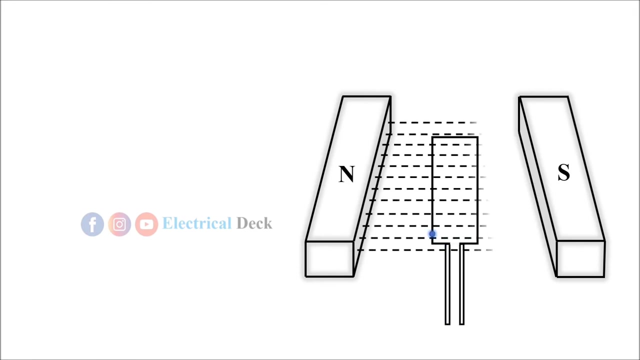 Z is equal to total number of conductors present in the armature And A is equal to number of parallel paths in which Z number of conductors are divided. Now, when the conductor is rotating in, the magnetic field, EMF, gets induced in the conductor. 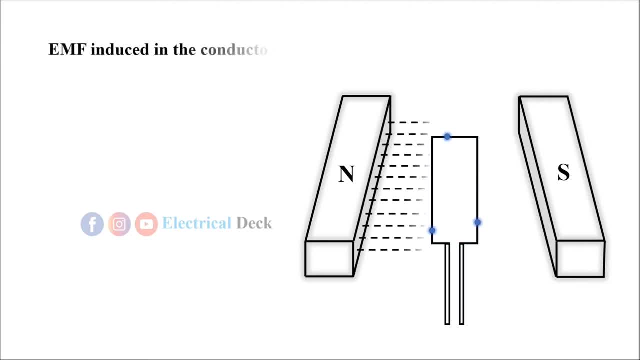 The amount of EMF induced in the conductor is given by E is equal to rate of change of flux, That is d pi by dt. Now, here, in one revolution, armature cuts the total flux produced by all poles, That is, change in flux. d pi is equal to total flux, pi into total poles, P. 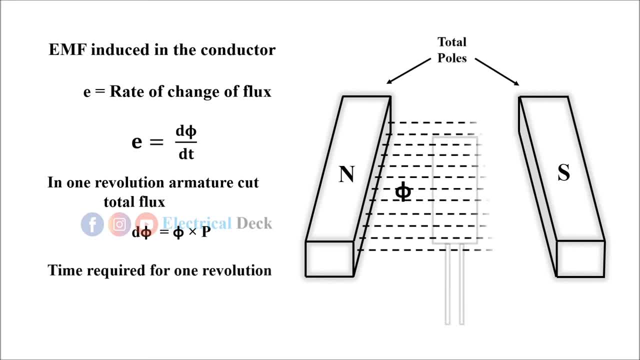 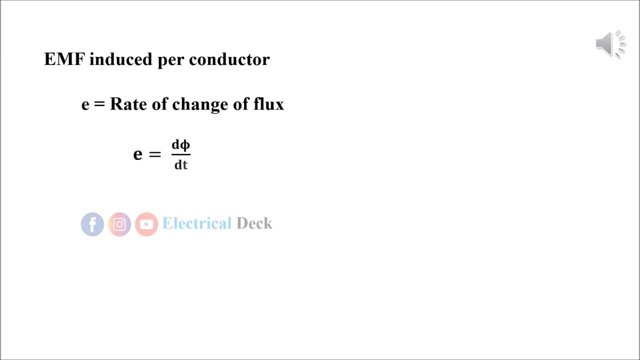 And the time required for armature to complete one revolution is given by. dt, is equal to 60 by speed of armature. N From the equation of EMF induced in conductor, that is d pi by dt. d pi is equal to pi into P. 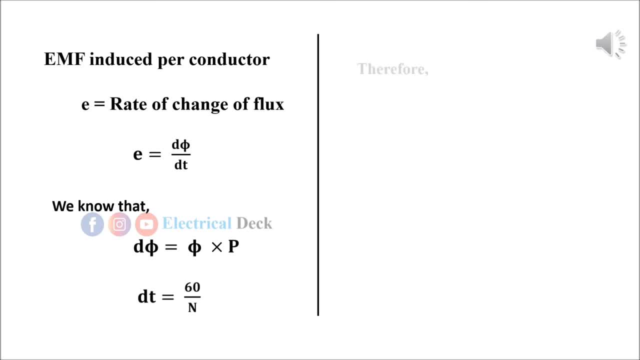 And dt is equal to 60 by N. Therefore, by substituting the values we get EMF induced per conductor. E is equal to pi, P, N by 60.. Now we know the equation for EMF induced per conductor, That is, EMF induced in only one conductor. 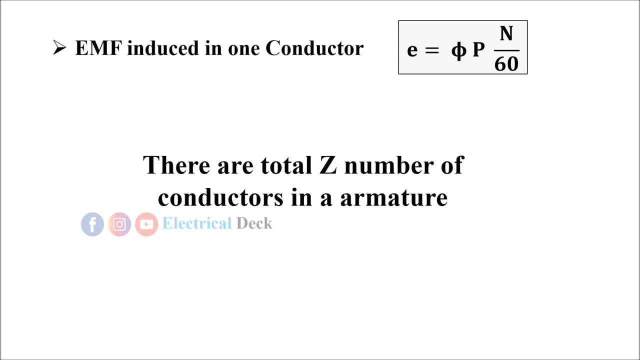 And we know that there are total z number of conductors in the armature. But in a DC generator the conductors in one parallel path are always in series. If there are total z conductors and a parallel paths, then z by a number of conductors are always in series.